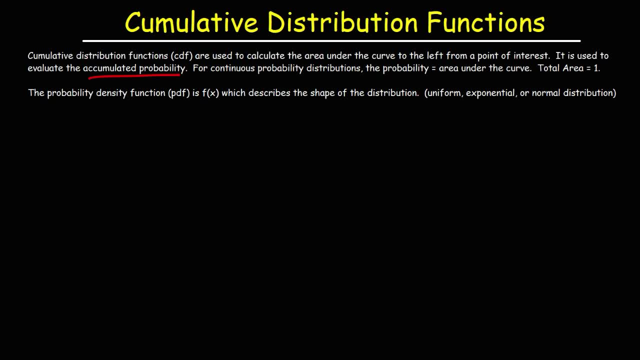 that wrong. the accumulated probability Now keep in mind. whenever you have a continuous probability distribution, the probability is equal to the area under the curve, And since the maximum probability is 1, the total area under the curve will be 1 as well. Now, probability density functions are: 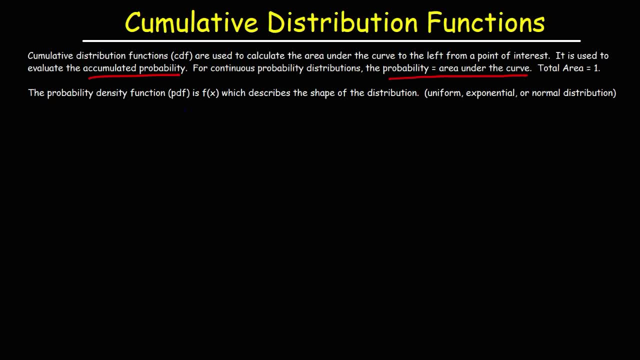 different from cumulative distribution functions. The PDF or probability density function is f of x and it's helpful to know that the probability density function is f of x. and it's helpful to know that the probability density function is f of x and it's tells you the shape of the distribution. So, for instance, let's say if we have a 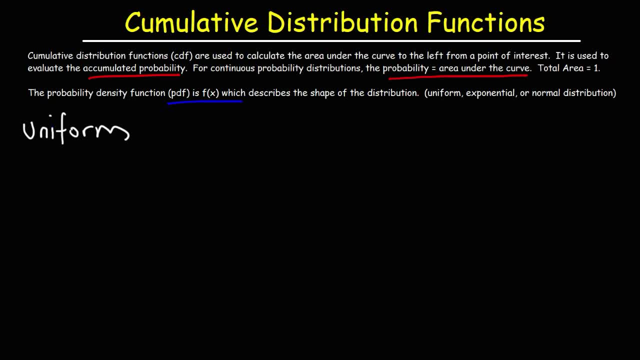 uniform distribution. In this case, f of x will equal a specific number. It's going to be a constant value. F of x is going to be 1 over b minus a. for uniform distribution. It's a number. It doesn't have the variable x in it. 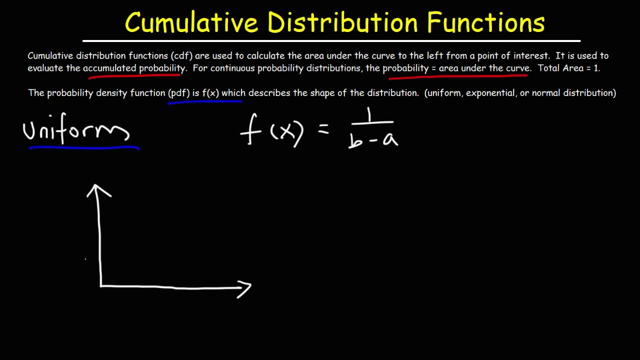 You'll see something that looks like this: So this is f of x and it varies from a to b. So this right here is the PDF, That is the probability density function. for a uniform distribution, It's equal to f of x. Now the CDF. 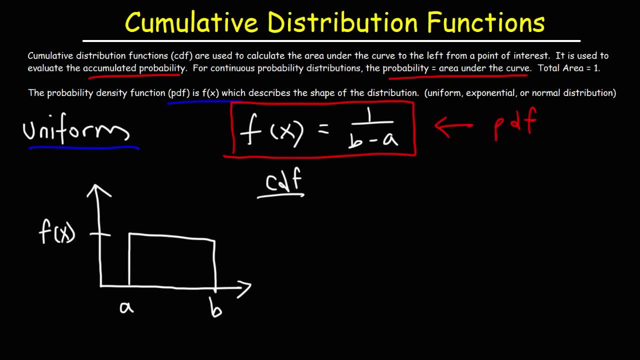 the cumulative distribution function will give us the area under the curve to the left. So let's say the point of interest is x. The CDF will give us the area to the left of x, So the area of the shaded region in blue. Now this is. 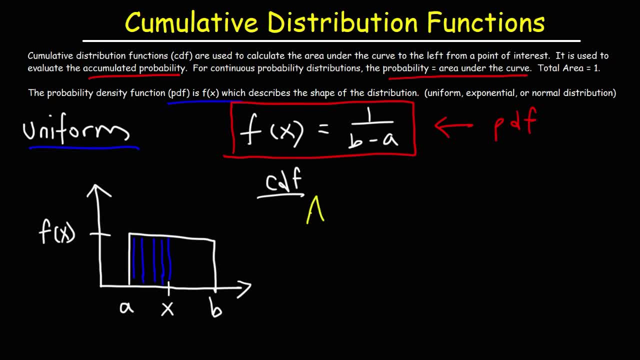 basically the shape of a rectangle. The area of a rectangle is the base times the height. Notice that the base is the difference between x and a, So it's x minus a. The height is f of x, And f of x is what we see here: b minus a. So the CDF, the 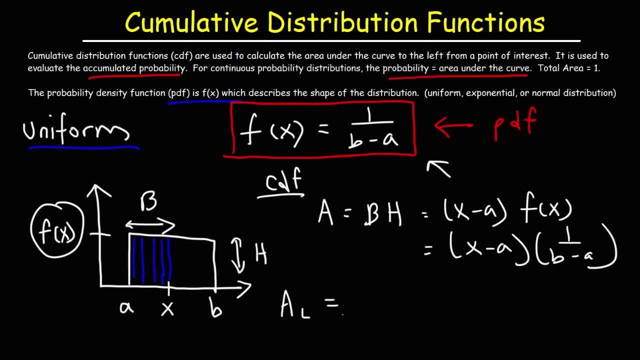 cumulative distribution function will give us the area to the left. So we have this formula: The probability that the random variable capital X is less than or equal to some number is going to be X minus A over B minus A. So this function right here highlighted in blue, this is the CDF. 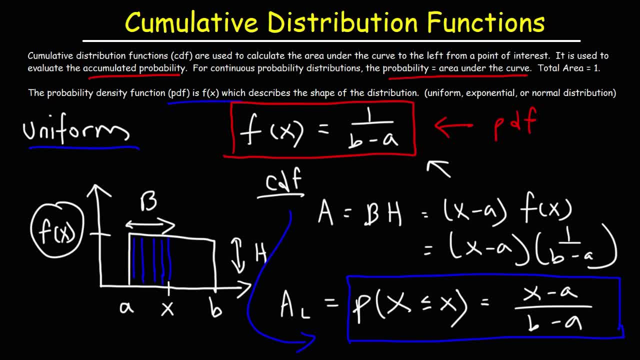 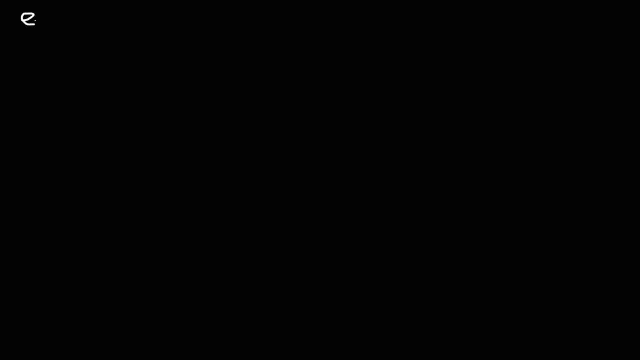 That is the cumulative distribution function. for a uniform distribution, It gives us the area to the left of some value, X, And the PDF is just F of X. For uniform distribution, that's 1 over B minus A. Now let's talk about the exponential distribution. 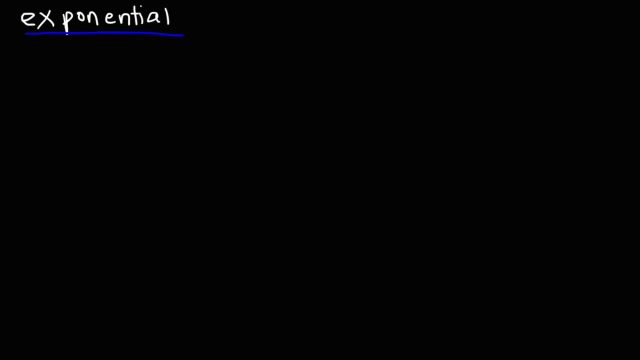 Let's discuss the CDF and the PDF for this type of distribution, The exponential distribution. The maximum value is the y-intercept and it decreases over time. The maximum value is also known as lambda, the rate parameter. The probability density function for an exponential distribution is going to be the function F of X. 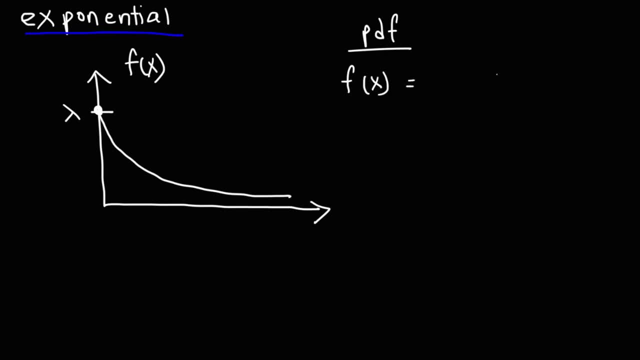 which describes the shape of the distribution, And F of X, for this particular distribution is lambda. E To the negative lambda times X. And lambda is the rate parameter. It's 1 divided by the mean. So this is the probability density function. 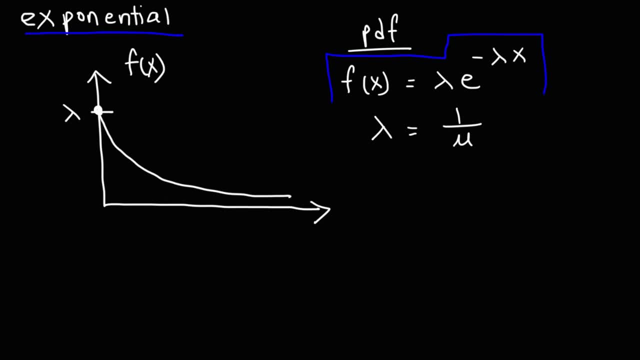 It tells you the shape of the graph. That's what it does. In addition, it also gives you the height of the curve above the X axis at some point X. That's another thing that it tells you. Now the CDF gives us the area under the curve to the left of some value X. 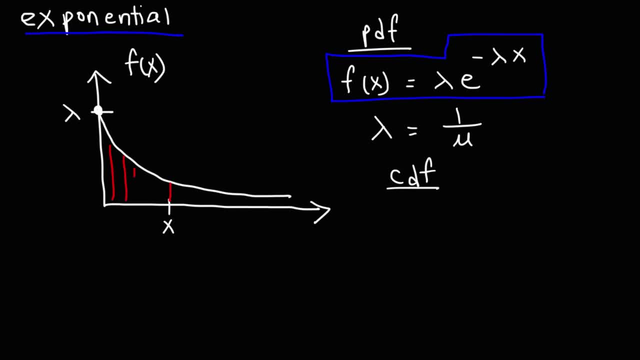 So let's say, if we wish to calculate the area to the left, So that's going to be AL, That's going to be the probability that X is less than or equal to some value X, and that's going to be equal to 1 minus e, to the negative lambda times x. 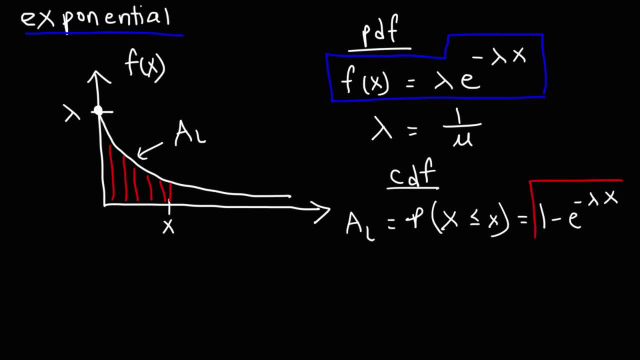 So that is the cumulative distribution function. It gives us the area under the curve to the left. So if we wish to calculate the probability that x is between 0 to x, or let's say 0 to a, this function will help us to get the probability. 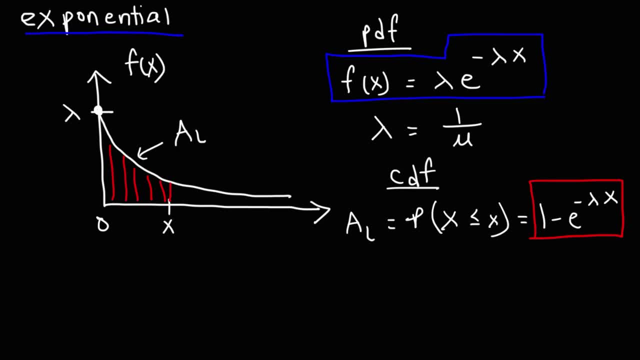 It's equal to the area under the curve. Now what if we wish to calculate the area to the right as opposed to the area to the left? We know that the total area is 1.. So the area to the right plus the area to the left must also be 1.. 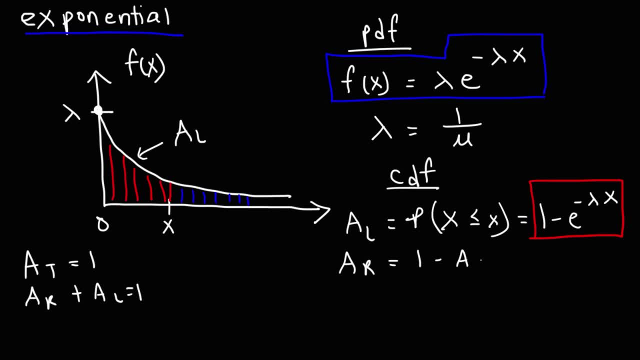 So the area to the right is 1 minus the area to the left, And we know the area to the left is what we see here. It's 1 minus e to the negative lambda times x. Now, if we distribute the negative sign, 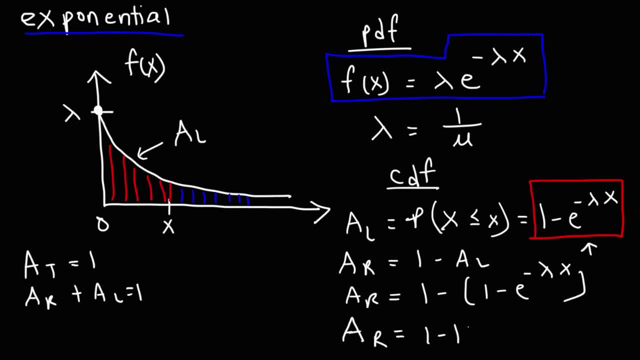 that is this negative sign. it's going to be 1 minus 1 and then these two negative signs will cancel, giving us a plus sign. So plus e to the negative lambda times x. So 1 minus e to the negative lambda times x. 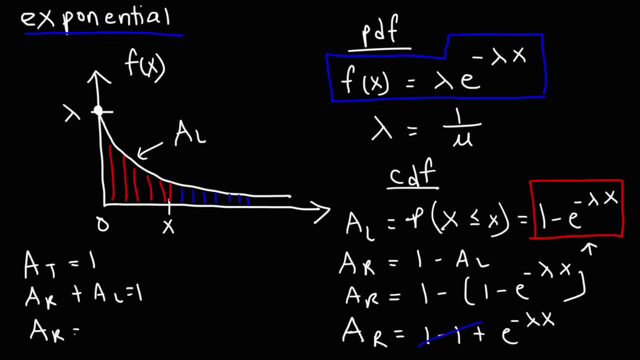 1 minus 1 is 0. Thus the area to the right is going to be simply e, to the negative lambda times x. Now, this is not the cumulative distribution function, because it doesn't give us the area to the left, It gives us the area to the right. 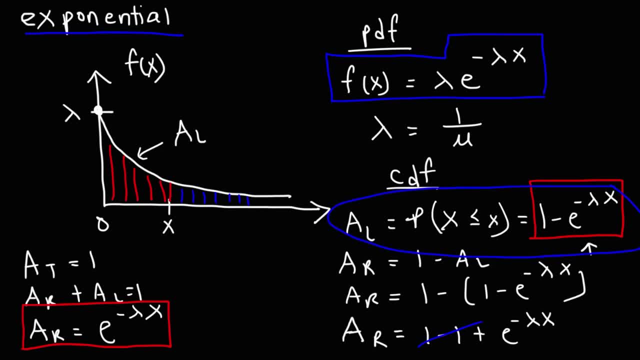 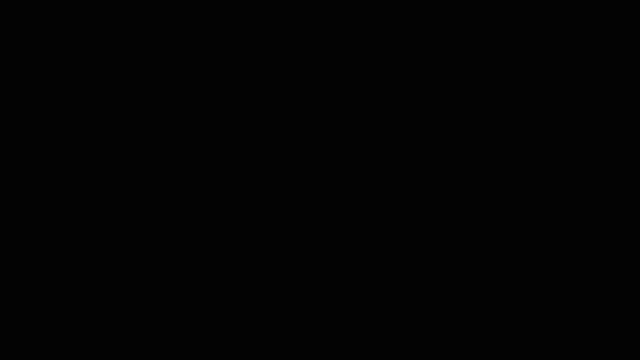 So the CDF is what we see here, That's the CDF for an exponential distribution. Now let's say if we still have an exponential distribution. but we want to calculate the area between a and b. So we want to find a probability that x is somewhere between a and b. 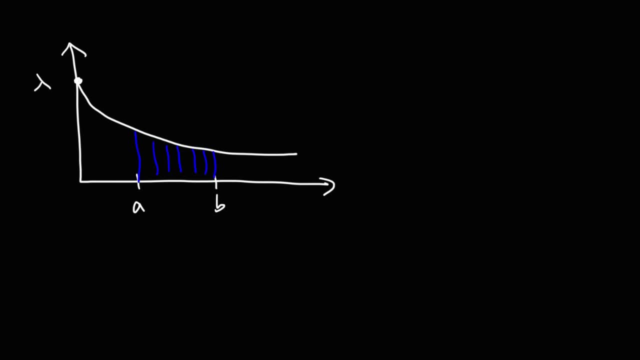 How can we calculate the area under the curve between those two points? So this area highlighted in blue is equal to the probability that x is somewhere between a and b. So we want to calculate the area under the curve between those two points. x is between a and b And that is the difference between the probability that x is less than b. 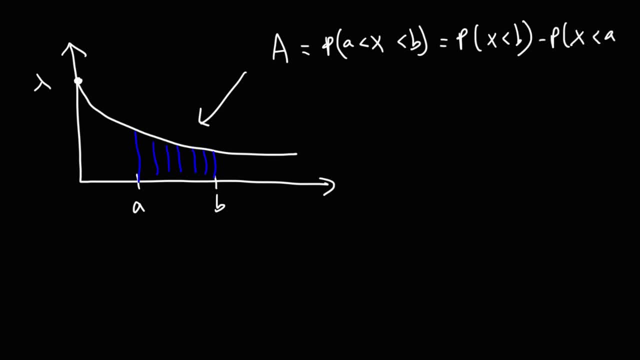 minus the probability that x is less than a. So these are areas to the left. So we could use a CDF to calculate the probability that x is less than b and the probability that x is less than a. The probability that x is less than a would be the area shaded in red. The probability that x. 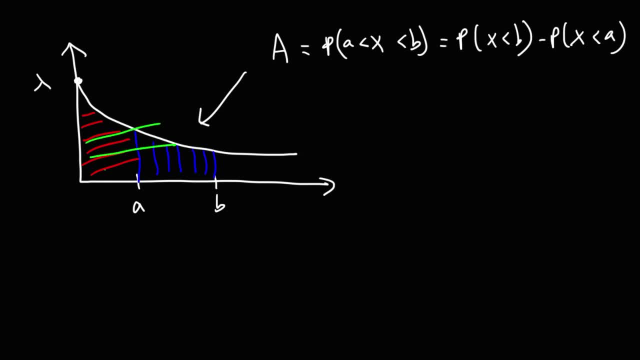 is less than b would be the area shaded in green. If you subtract the area shaded in green minus the area shaded in red, you'll get the area shaded in blue. So using the CDF function, we can replace that value with. this is going to be 1 minus e to the negative lambda Instead of x. 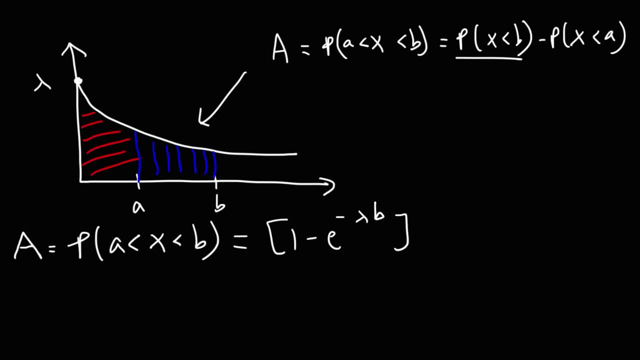 we're going to replace x with b, So this will give us the area to the left of b. Now we need to use the CDF function to get the area to the left of a, And that's going to be 1 minus e. to the negative lambda times a. 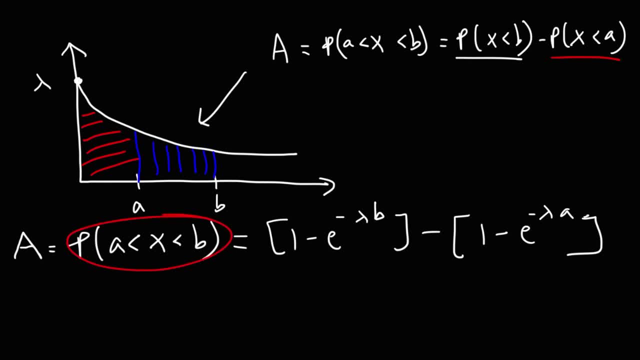 So this is how we can calculate the probability between a and b using, or if we have, an exponential distribution. Another thing that you want to keep in mind is that, for a continuous probability distribution, the probability that x is greater than or equal to a, or and rather less than or equal to b. 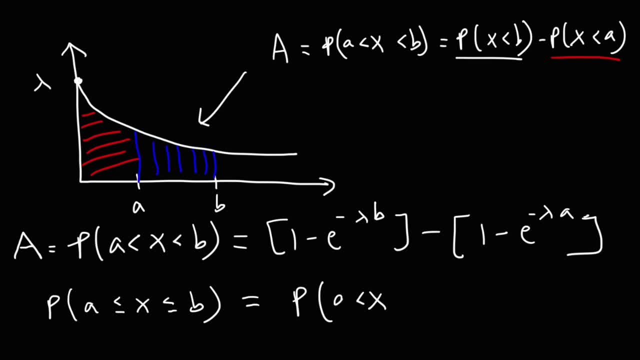 this is the same as the probability that x is between a and b, So you want to keep that in mind. There's no difference here. Another thing that you want to keep in mind when dealing with continuous probability distribution functions is that the probability that x is a single value as opposed to an interval of values. 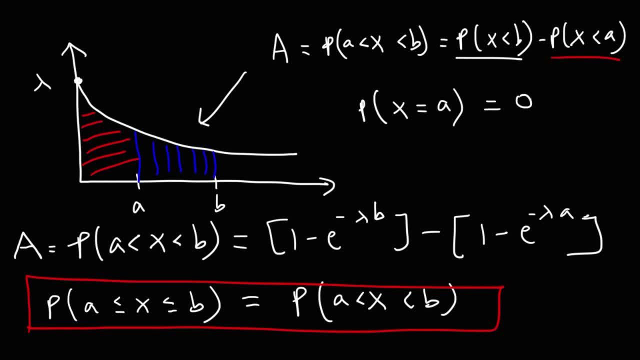 let's say the probability that x is equal to a, that's going to be 0.. The only way to get a value greater than 0 is you need a range of x values, Because at x equals a, all you have is a line. 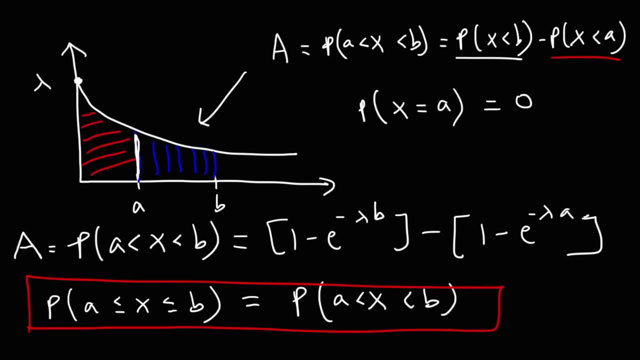 You can't really calculate the value of a line. You can't really calculate the value of a line. You can't really calculate the value of a line. You can't really calculate the area of a line, Because you have height but there's no width.